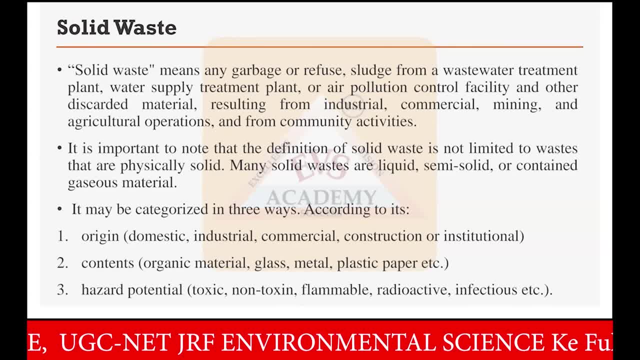 the name. it is a kind of solid and solid that is not in use or that is we need to dump. that is the solid waste and it is containing, or it is having all the things which are the garbage or refuse or maybe sludge from the wastewater treatment, which is left after removing all the water. 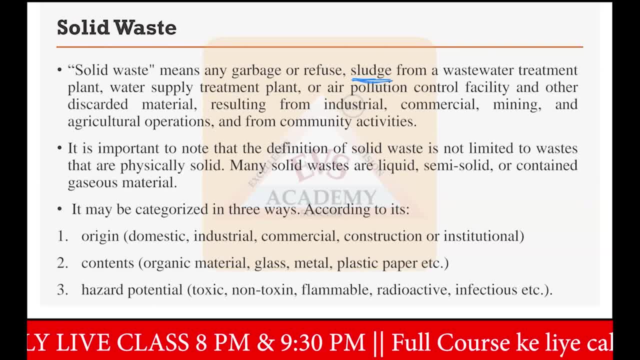 So that solid pores. the solution of the wastewater is sludge and water supply treatment plant, that solid things coming out from the water supply treatment plant, the air pollution deposition or the particulate matters we are getting after the purification of air control facility and other discarded 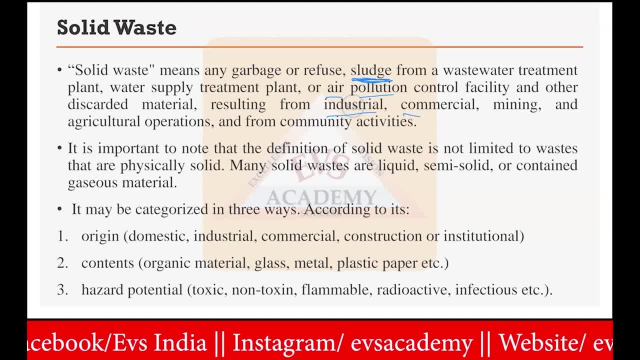 material resulting from the industrial processes, maybe commercial processes like building materials or the demolishing things. Those are the commercial solid waste. Then we have the mining materials and the agricultural operations and from the community activities. So all that solid form of wastage are under the solid waste category. It is important to note that the definition of solid 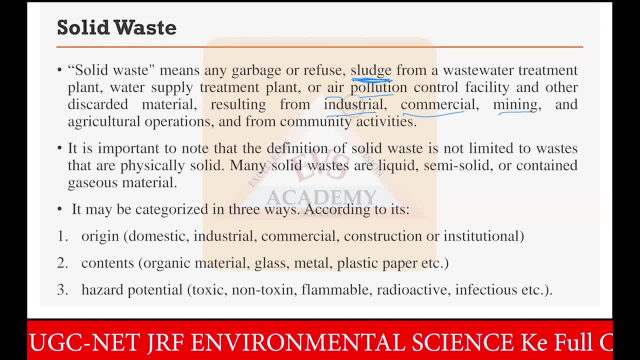 waste is not limited to the wastage that are physically solid. It is not necessary that waste should be only and only solid. The wastage material can be liquid as well, the semi solid as well, And it is containing some gaseous material as well. that all the things are under the category of. 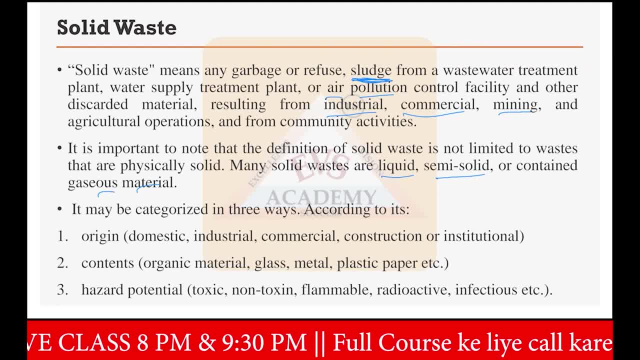 solid waste. Do not assume that all the solid waste are solid in nature. These can be semi solid, liquid or gaseous as well. If you look at these solid wastes, you can categorize them in the three different categories according to its origin. that you can again define the particular types of the solid. 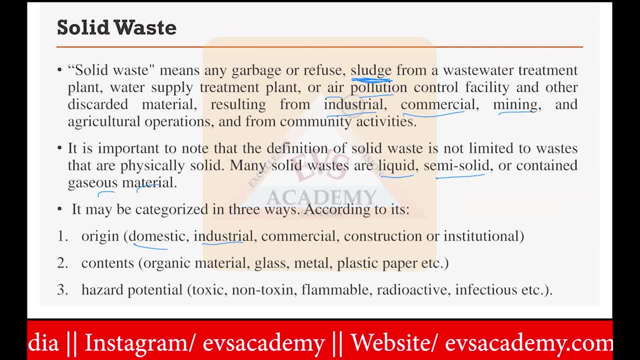 waste here The domestic type of solid waste. we have industrial type of waste. You can have commercial type of waste- construction and the building material- or maybe institutional type of solid waste You can have under the category of solid waste based on the origin of the waste, from where that particular? 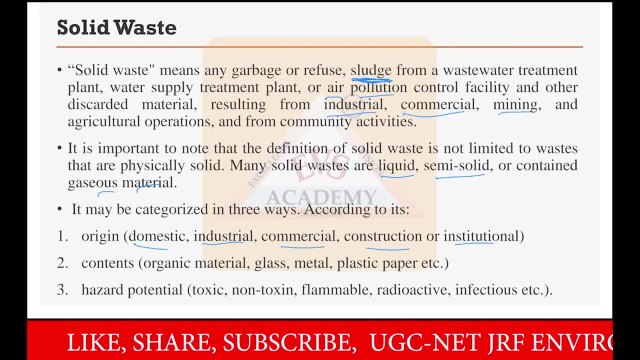 waste is coming, Then according to the content of the waste, again, you can define this waste in multiple categories. Worst category here can be the organic material waste, glass material waste, then metal waste or plastic, paper waste. Anything is possible that all under the different category of the solid waste. 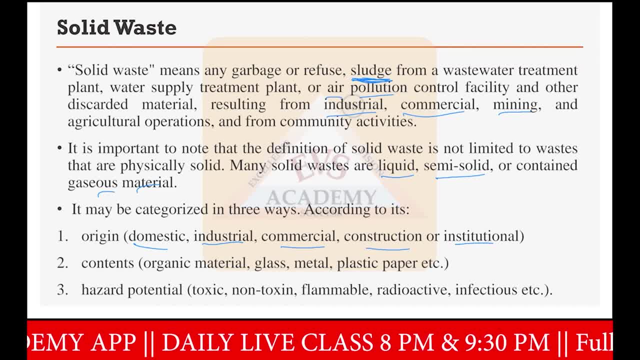 based on the content of that particular waste, Then according to the hazard category you can define the category of solid waste. based on the origin of the waste, Then how much toxic it is to its origin, how much hazardous the particular waste. according to that again you Can classify it under the multiple categories like toxinöm. 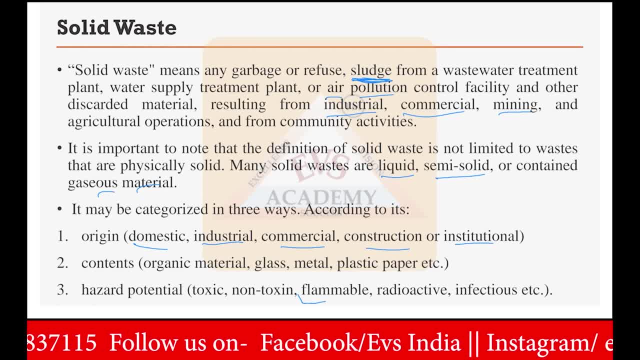 elements, surfaces, non-toxin items. flammable, which is the pattern of waste which is ready to take fire very easily, ie the flammable type of solid waste radioactive, from which radioactive in the לא�e waves, Maybe an Alpha matter with an alpha beta radiation, is coming out, ie an radioactive menos radiation. 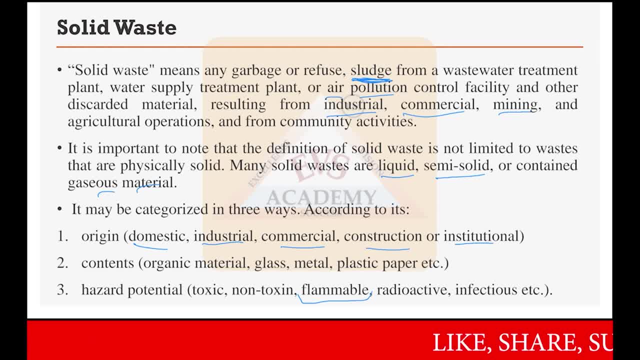 type of solid waste: Infectious solid waste which can cause any disease problem in the different organisms or in the human beings. those would be infectious solid waste, For example the waste which is coming out from the hospital or maybe from laboratories. so those all are kind of. 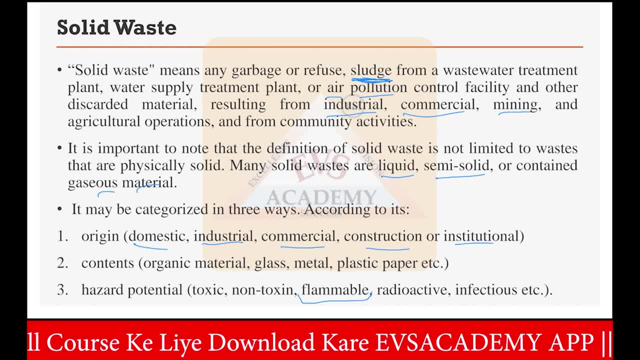 infectious solid waste. So under this particular chapter we have to study the nature of these different solids waste. that is the first thing. Another thing: what are the solutions of these different solid wastes that we have to discuss? and the third thing that we have to discuss is: 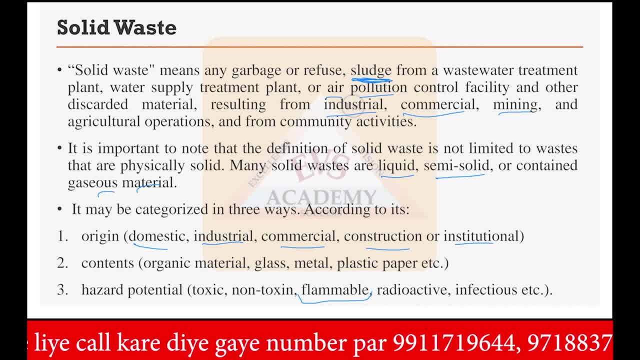 the different laws and regulation, rules and regulations under which you can just decompose these different solid wastes. So all that thing we have to discuss in this particular unit- and that's all about this particular unit- is: So let's see, the first thing that we have to discuss here. 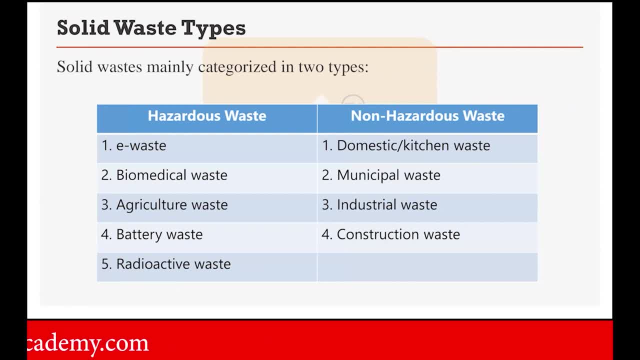 in the solid waste is the types of the solid waste. So the mainly solid waste is categorized in two different types. First is the hazardous waste. The handling of the hazardous waste is little bit different as compared to the non-hazardous waste. So second category we have here is the 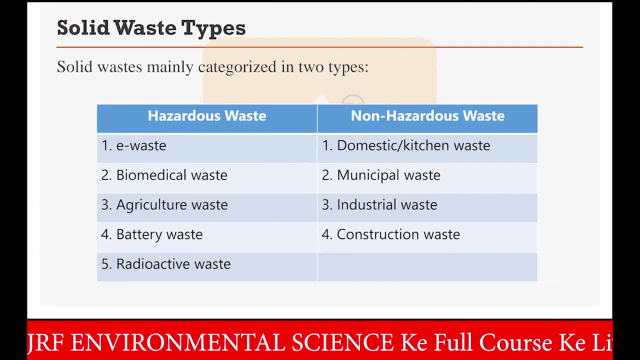 non-hazardous waste. In the hazardous waste we have e-waste, E-waste or you can see electronic waste which is coming out from the multiple electronic equipments. that is the e-waste. Biomedical waste, biomedical waste, that waste which is coming out from the laboratory, maybe. 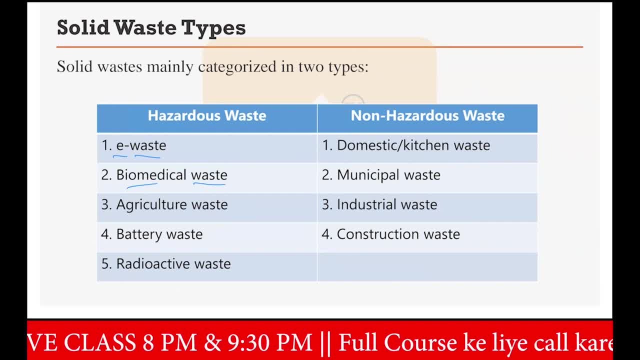 hospitals. that is, the biomedical waste, Agricultural waste that is coming out from the agricultural operations, Battery waste which is directly coming out from the battery, because battery is having multiple harmful elements in it like mercury, cadmium, nickel, zinc. these all materials you can find out in the batteries. 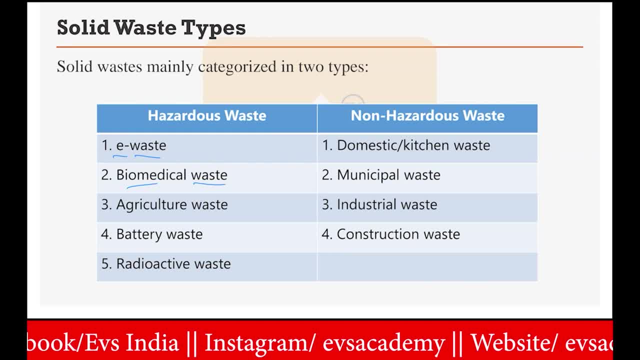 Then radioactive waste, from where the radiation is caused by any particular waste material, Maybe alpha, beta, gamma, and it can ultimately lead to the multiple disease problem and harm to the environment. Those are under the category of radioactive waste, which is under the category of hazardous waste. 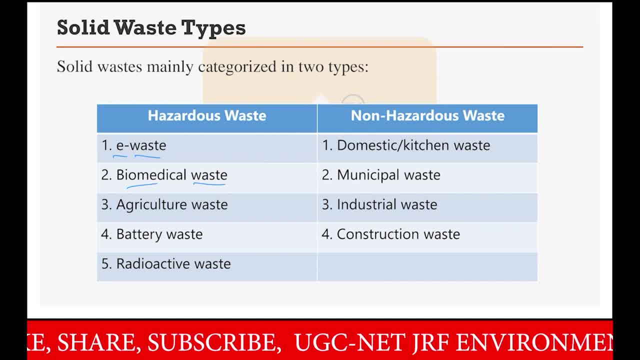 Then we have the non-hazardous waste, for example domestic or kitchen waste which is coming out from the household operations. So those all are under the category of domestic and kitchen waste. Then we have the municipal waste, and municipal waste- papers, plastic and those kind of different. 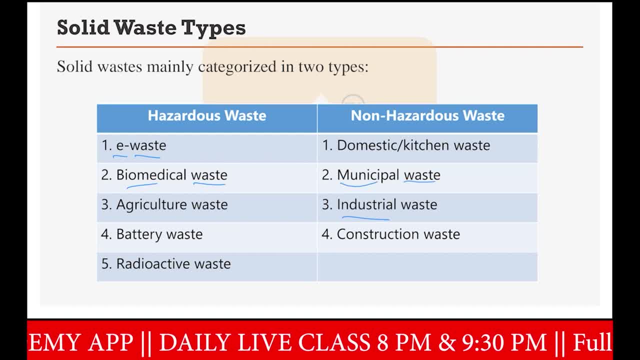 materials you will have in the municipal waste. Then we have the industrial waste that is coming out from any particular type of industry Only: construction waste, for example building materials, cement, and then the different raw materials of the building that is coming out from the destruction of the building. 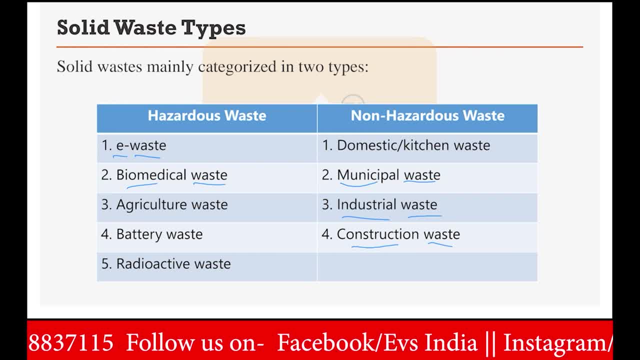 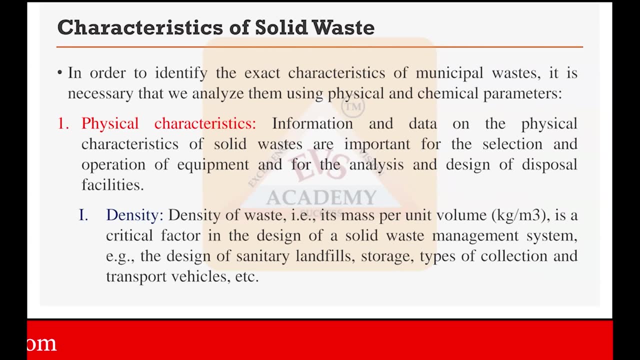 So those all are under the category of construction waste, which is again a type of non-hazardous waste. So these two are the main category of the different type of waste. Now we have to discuss how to know which type of waste is having what property. So here we have to discuss the 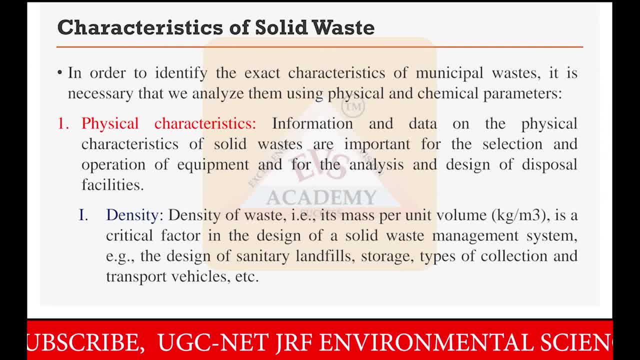 characteristics of the different type of solid waste. So in order to identify the exact characteristics of the municipal wastage, it is necessary that we analyze them using physical and chemical parameters. So here in the characterization process, we have to discuss about the two main parameters. 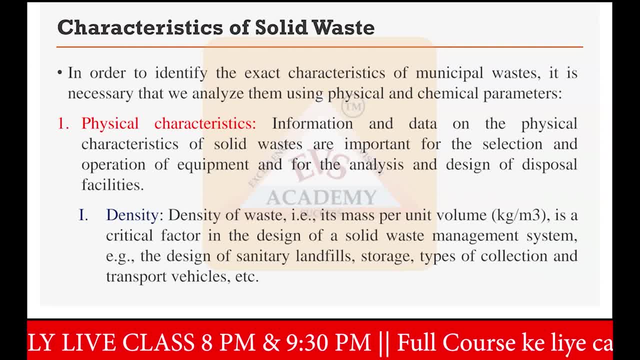 The first parameter here would be the physical parameter. The second parameter here we have to discuss that is the chemical parameter. In physical parameter we will see that all the physical characteristics like density and all that physical characteristic of any particular material. and in the chemical parameters we have to see what is the pH, what is VEC, what is the chemical? 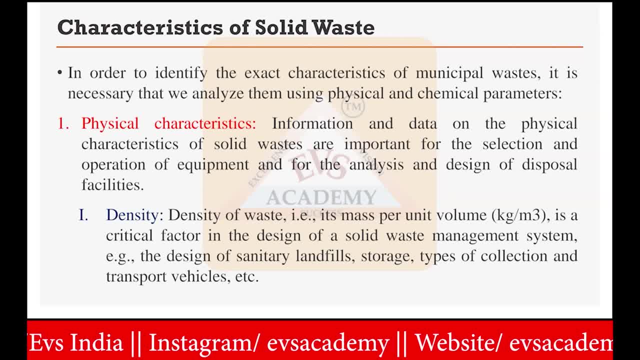 characteristics of that particular type of solid waste. So first we will discuss here the physical characteristic of that particular solid waste. So information and data on the physical characteristics of the solid wastes are important for the selection and operation of the equipment- this is important- and for the analysis and design of the disposal. 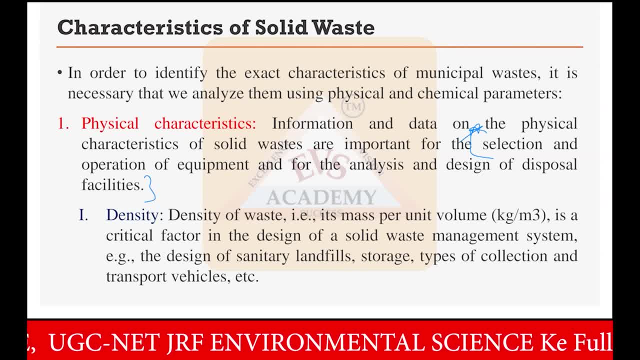 facilities. so according to that, the physical characteristics, whether it is a liquid material, whether it is a solid material, whether it is mixture of that, according to that you have to design your equipment and you have to design your disposal facility. so that is very important. that's why we have to study the physical characteristic of any particular type of solid waste. 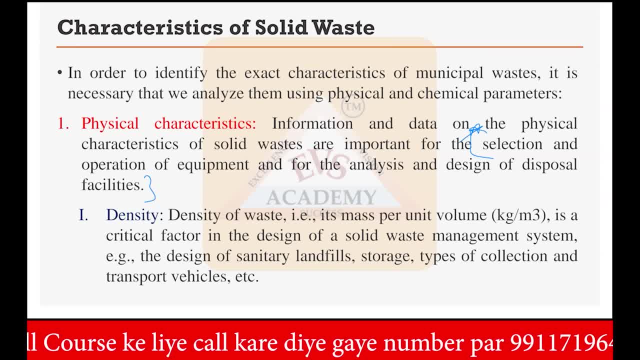 under the physical characteristics also, we have multiple categories that we have to discuss. the very first category under the physical characteristics is the density- density of the material. so the density of the solid waste is mass per unit volume, that is, kg per meter cube. that we have to find out whenever you are disposing or maybe operating with the solid. 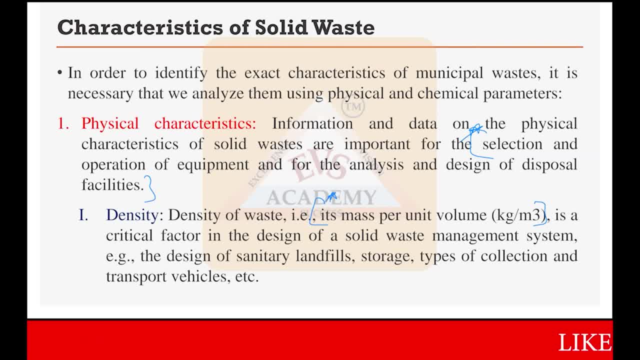 waste material. that is a critical factor in the design of the solid waste management system, for example, the design of the sanitary landfills. sanitary landfills means land fields, landfills. i think you know what is the landfills. landfills are the area, or maybe a dump. 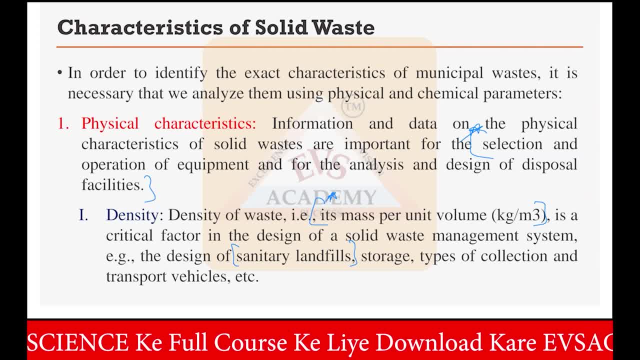 site where all the wastage material are dumped or all the wastage material are left there for the degradation process. so those are the landfills. landfills you have seen in the municipal cities or that metropolitan cities, the large heels of the landfills you can see there because of the excess. 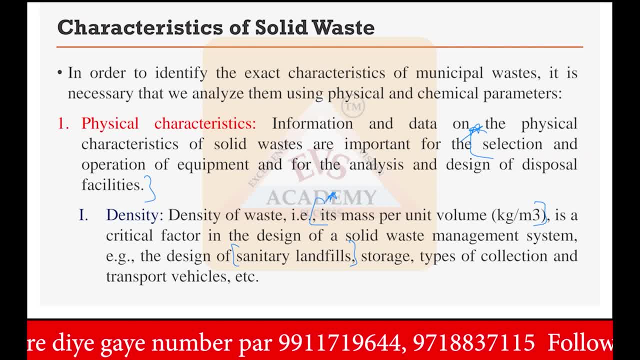 amount of waste generated there and the unavailability or lack of the treatment systems there. so those are the landfills. so landfills can be also of two types. one is the sanitary landfills, another one is the normal landfill that you have seen already. in sanitary landfills you have to design your landfills in such a way so it is not going to harm the 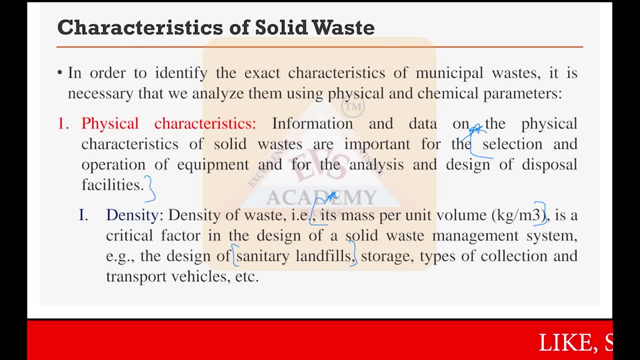 environment by any mean and ultimately that would be decomposed and mixed with the soil and it will provide a nutrition to the plant. so those are the sanitary landfills. in sanitary landfills you have to look at the multiple factors and parameters so it is not harming the environment and only 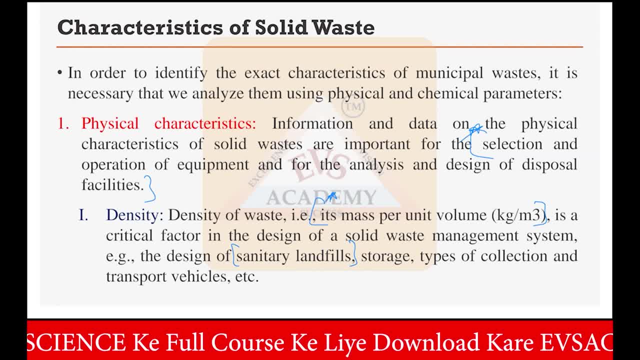 decomposing in its prescribed area. so those all are the sanitary landfills. sanitary landfills are generally not open. these are totally covered, maybe by the help of mud layer or soil layer. so the design of the sanitary landfills are very important and for that you should know. 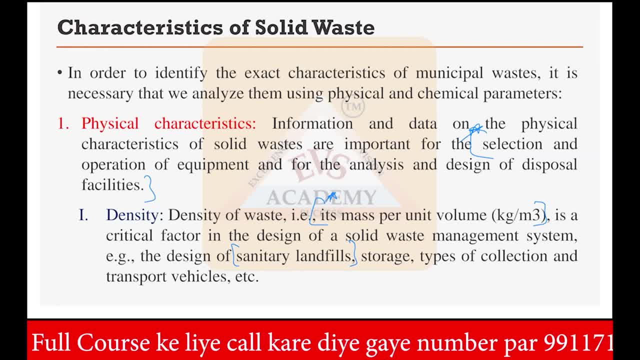 the density of the material. what type of materials are there? for example, you cannot dump plastic in the sanitary landfills because plastic is not going to decompose there, so only the biodegradable materials you have to use there. then suppose you want to store the wastage material in any. 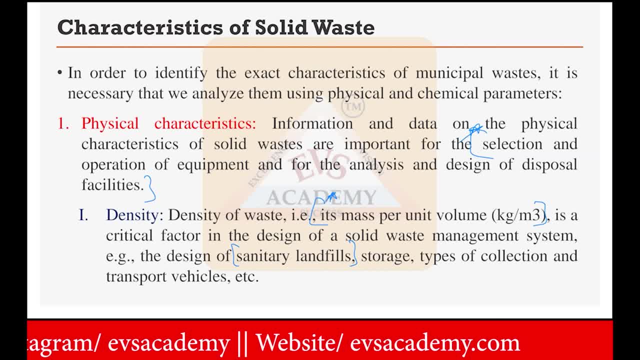 particular site for the time being. so for that also, you should know the density, types of collection and the transport vehicles that we need to use. for that also, we should know the density of solid waste. according to that we can design our collection system and the transport vehicles as well. so these all things are generally helped by 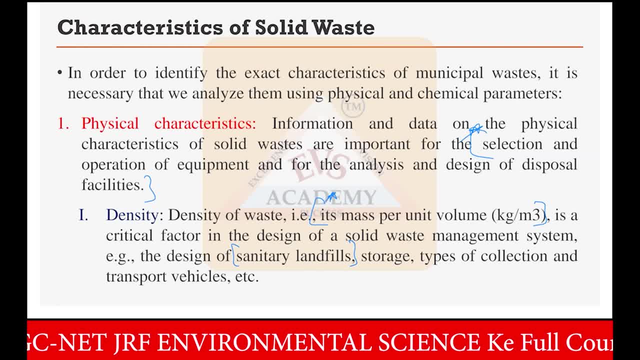 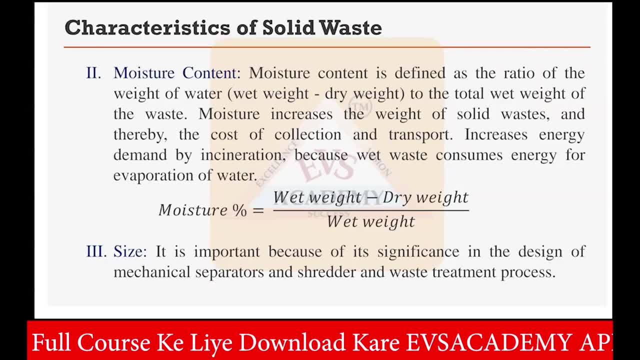 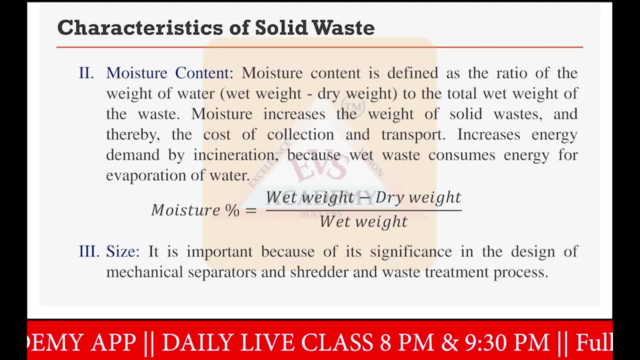 knowing the density of the waste material. so that is the first physical characteristic that you should know about the solid waste. the second very important characteristics that you should know about the solid waste is the moisture content present in the solid waste. for example, a particular biomedical waste is having very high moisture content. that is not. 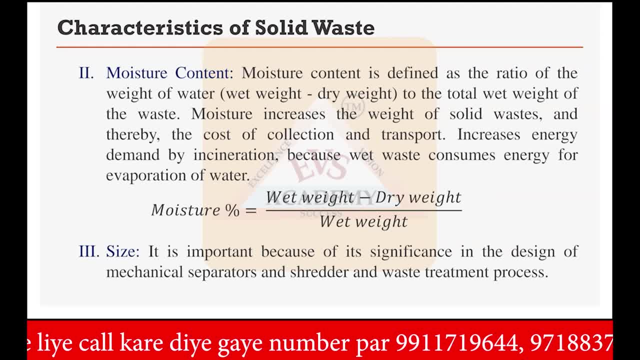 suitable for the incineration. what is incineration? incineration? incineration process is done in the equipment called as incinerators. these incinerators have a kind of volume. there we are where you have to put your all solid waste or the wastage material and then the decomposition takes place in very high 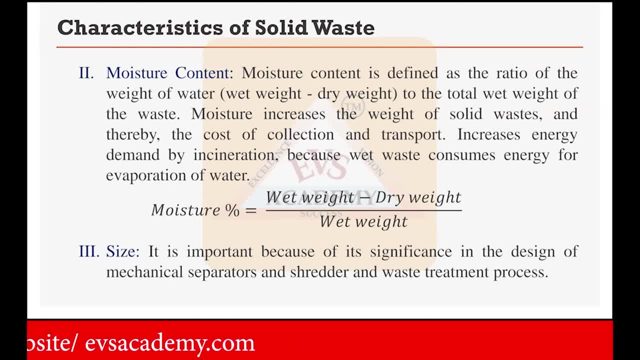 temperature. so ultimately what you are doing, you are just burning the materials here. so if your materials are having very high moisture content, so those things are not suitable for the burning process or incineration process. so first you have to remove the moisture, or it should be in the 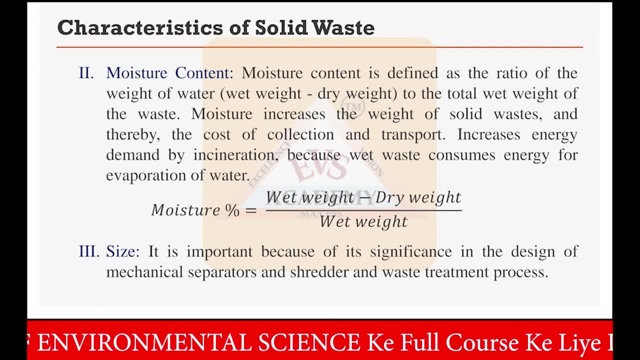 limited amount, then only you can go with the incineration. so that's why the moisture content analysis is very important. the moisture content is defined as the ratio of the weight of water, so weight wet weight of that material minus removing all the water, you have to take the dry. 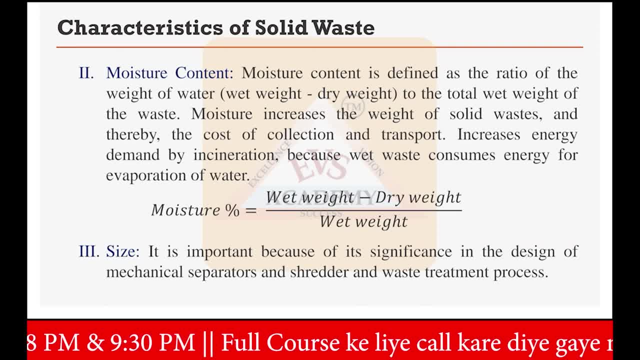 all the water. so that difference will give you the moisture content amount in weight. and if you once divide this weight with the total wet weight, so you will get percentage of the moisture content. after multiplying this particular thing with 100, from that way you will get the moisture percentage. 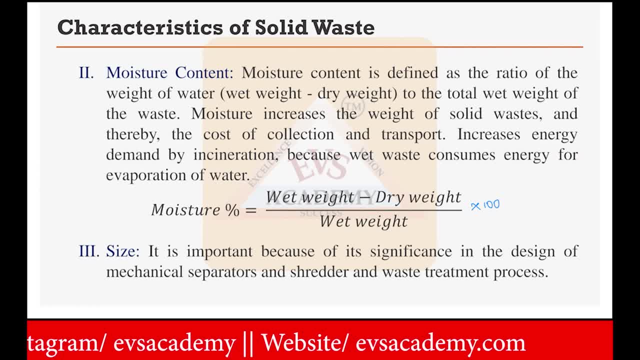 there. this moisture percent is telling that how much water is present in per 100 unit of that particular solid waste. suppose you have one kg of the solid waste and in the one kg there is a 100 gram of the water present in this so wet weight. when you will take you will get 1000 gram. 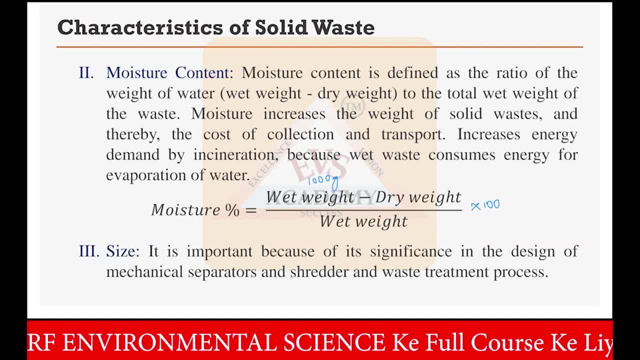 after drying that all the material, 100 gram water would be go away and only 900 gram of the material would be left. so 1000 minus 900 is equals to 100 divided by the wet weight. wet weight is equal to 100 gram of the water present in this. so wet weight, when you will take, you will get. 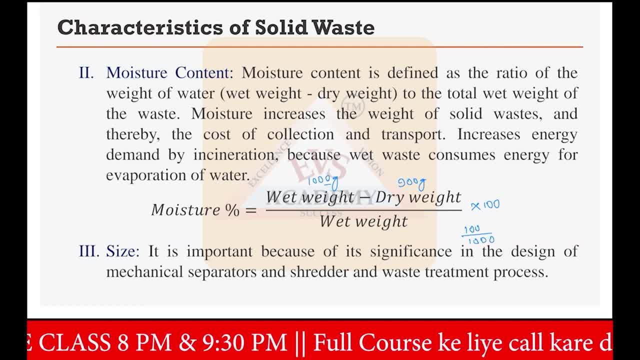 it will be 1000. that is the already measured weight that you have already measured. this is multiplied by 100. so this and this cancel, this and this cancel. then ultimately you are getting that in your waste material 10 percent of the moisture is present. so moisture increases the weight of the 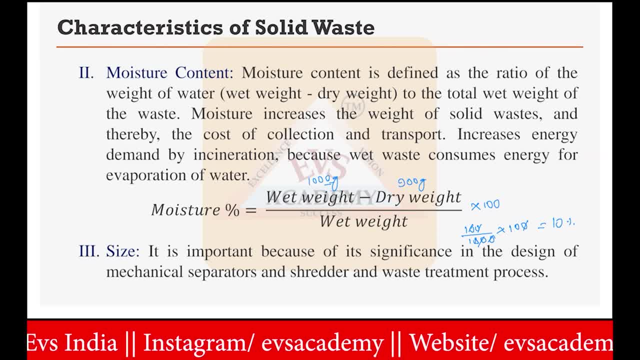 solid waste that you can see here earlier. the solid waste or dry weight, is only 900 gram, but 100 gram of water is added there. so it is increasing your weight of the solid waste and there why the cost of the collection and transport will also increase. so this content, moisture content, is 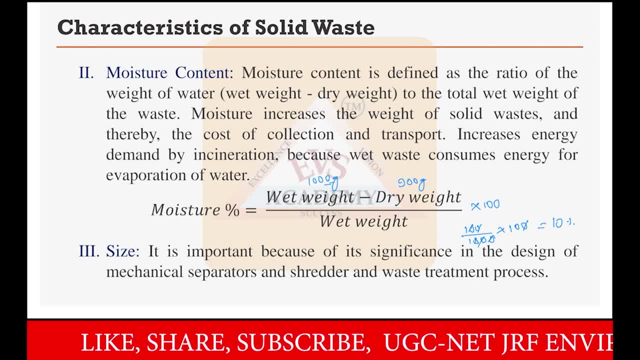 very harmful, you can say, in the terms of just disposing, collecting, transporting the wastage material. ultimately it is increasing your cost in all the things. it increases energy demand by the incineration. as i have told you, you cannot incinerate the content, which is having very high 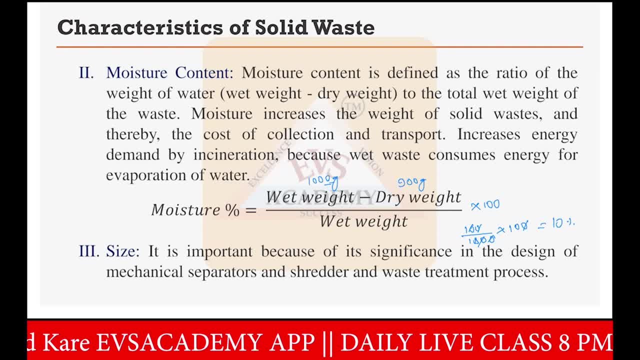 moisture content. otherwise there would be very high demand of energy by the moisture present in it. first you have to vaporize it, and then you have to vaporize it, and then you have to vaporize it, all the moisture present in it. once it is dried completely, then only you can burn it. otherwise 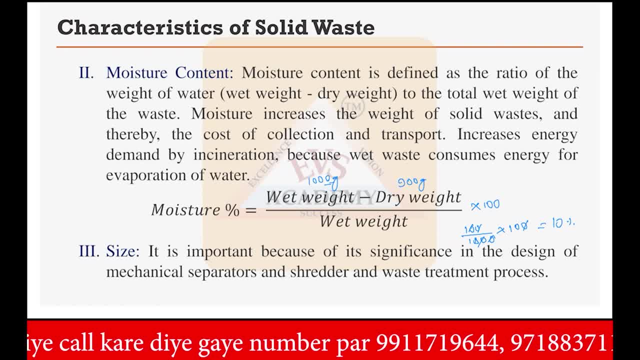 not. so that's why this is not good to have high moisture content in the incinerators for the waste test type in the incinerators, because wet waste consumes energy for the evaporation of water first and then it takes, it takes place the burning there or incinerating there. so this is all. 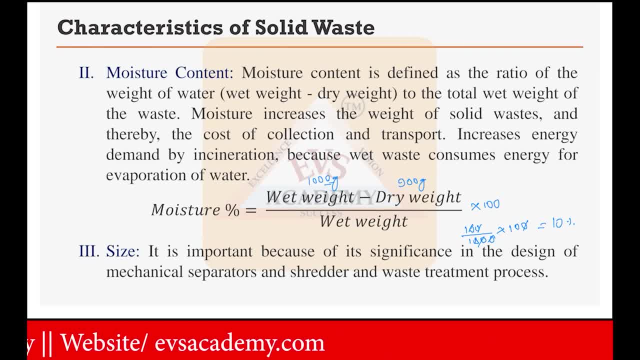 about the moisture content of the solid waste. you should also remember this formula also, so either hope it is clear to you. the next physical characteristic that we have to discuss here is the size of the material or the size of the solid waste. so it is important because of its. 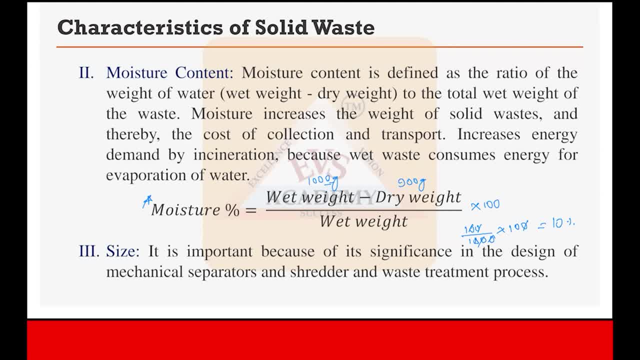 significance in the design of the mechanical separator and shredder. now, mechanical separator means that separator which is working in a machine or mechanized mode, that is, the mechanical separators. so suppose multiple type of mechanical separators are nowadays available. some are based on the laser beam, some of them are based on the moisture content. suppose you have a belt conveyor. 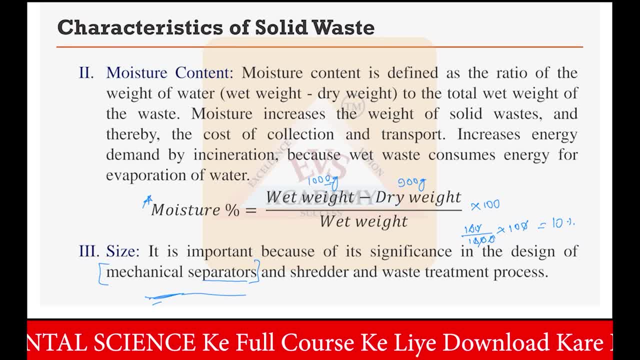 belt and you have ordered the machine that all the materials which is having more than 30 percent moisture- so those are materials- should be removed in this conveyor belts. the solid wastage will move ahead and there would be a scanner, maybe spectroscopy, maybe electromagnetic radiation based. so these will scan the materials and whenever it is. 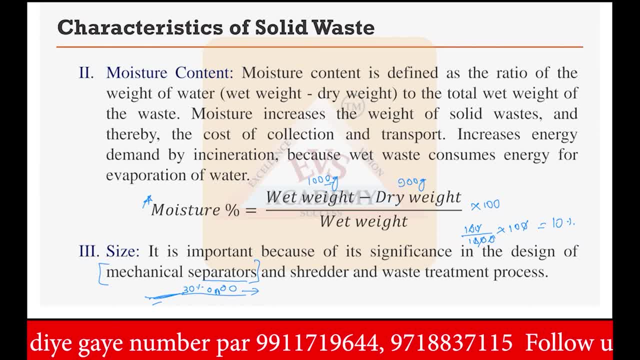 founding more than 30 moisture, immediately it will order the machine to remove that equipment. so there would be a arm here which will ultimately pull this material from out of the conveyor belt. so this is one example. suppose you want to just separate the plastic material? so again through. 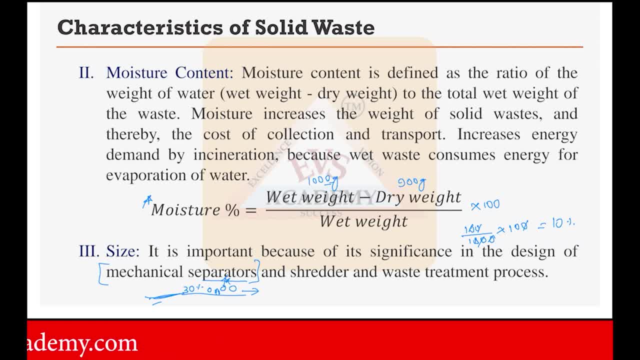 scanning you will get to know, the machine will get to know and with a harm arm separator it can remove easily all the plastics. presently that is a kind of mechanical separator. then shredder- what is the shredder? shredder here is used to just keep small pieces of a large 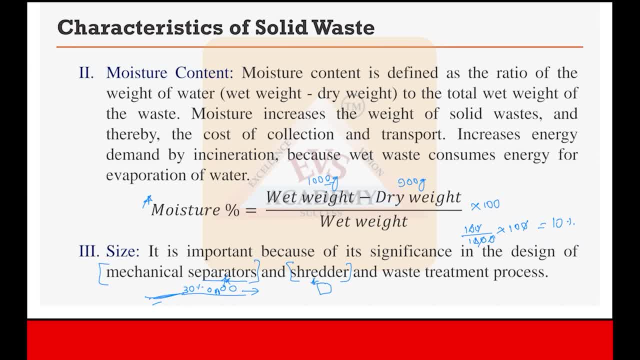 material. suppose you have a waste material which is of this particular size, but you want a smaller size of these materials. so what you have to do, you have to put this in the shredder and in this render you will get a small, small pieces of these particular solid waste which is crossed there in. 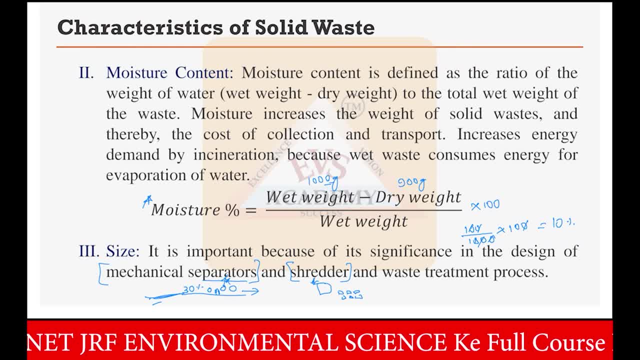 the shredder. so that is the work of the shredder. and if you want to do the shredding of the solid waste, so what type or what size of the shredder you want to use, that will depend on the size of the wastage material. if the size of the waste material will be very large, then large shredder.